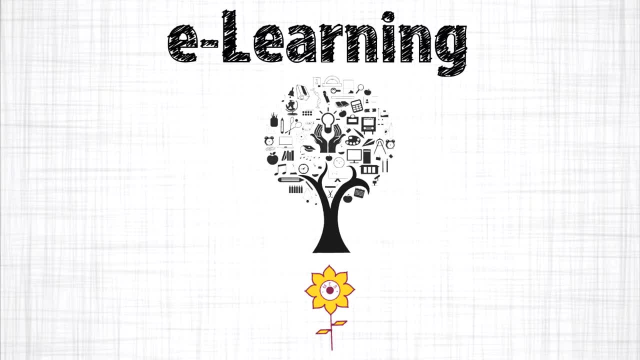 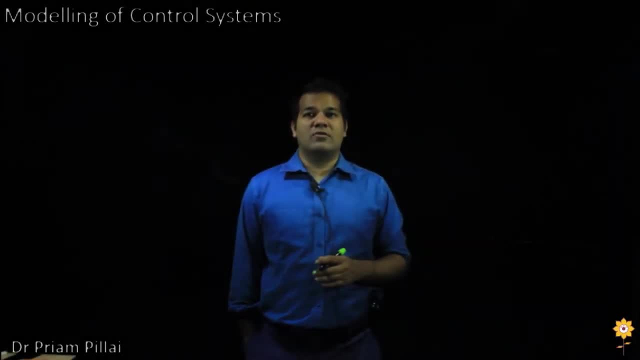 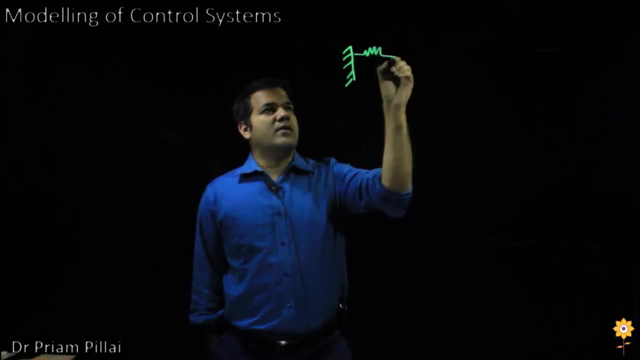 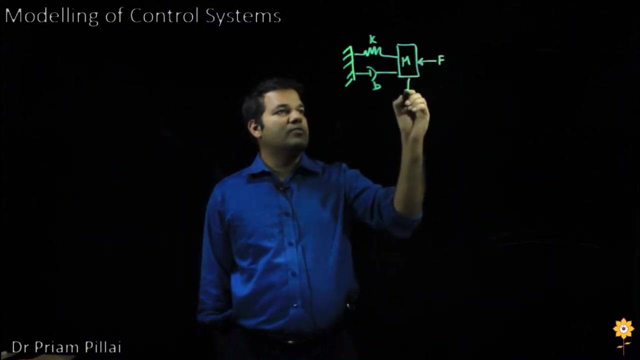 Today we'll be talking about how to create mathematical models of control systems. We'll start with considering a simple linear translational system having a spring, a mass and a damper. We apply a force F to this mass and measure its position x. We would like to write down: 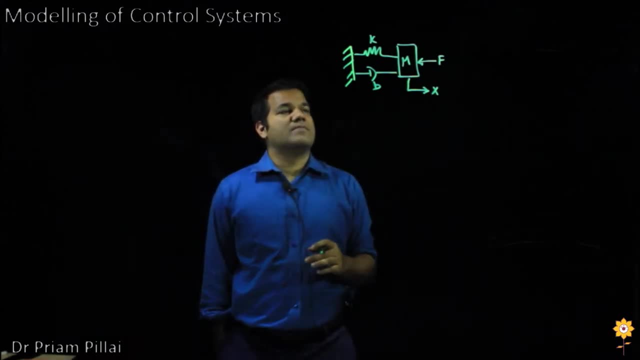 a simple mathematical expression that would govern the dynamics of this system, And we'll do so by applying Newton's laws. So consider this: mass m. According to Newton's laws, the sum of all the forces acting on that mass would be equal to the force F. So we'll 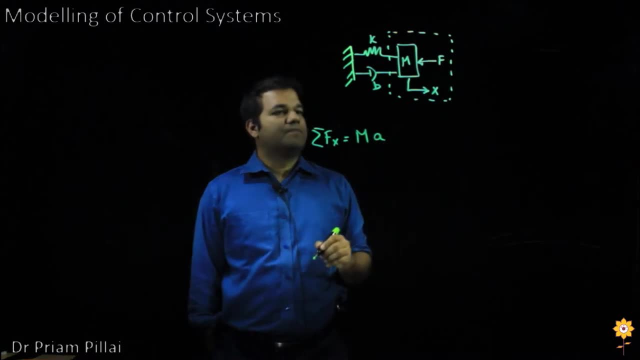 be given by the mass times its acceleration. And the acceleration is nothing but the second derivative of its position. The other forces acting on that mass would be given by the input force F. in the spring force, kx and its minus would always oppose the input force. 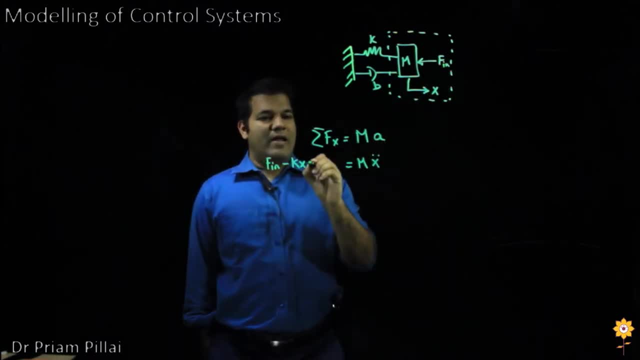 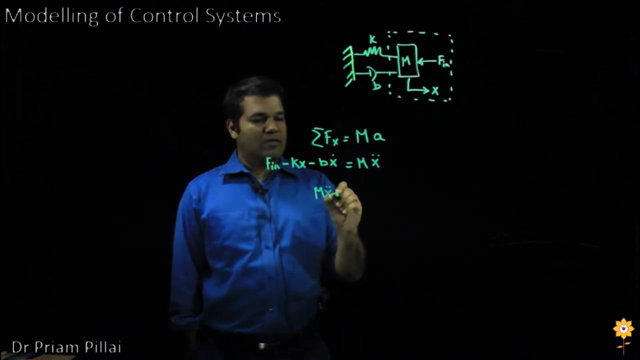 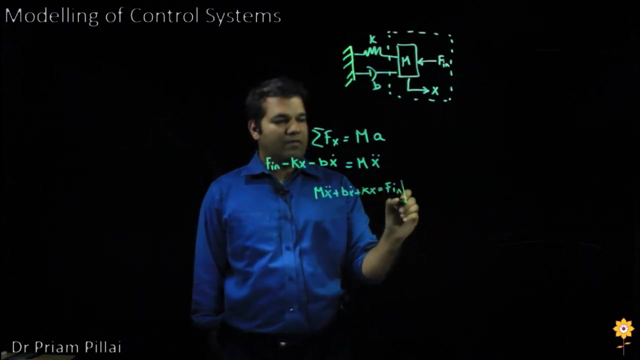 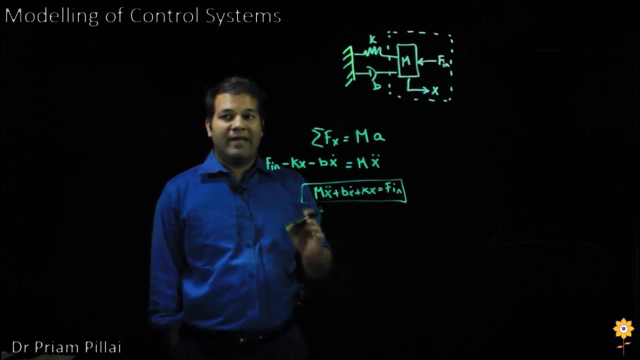 F in and a damping force That will be given by the damping coefficient multiplied by the velocity, which is x-dot. Rearranging all of this, we get m x double-dot plus bx-dot plus kx equals F in. This is a linear, second order, ordinary differential equation with constant coefficients. 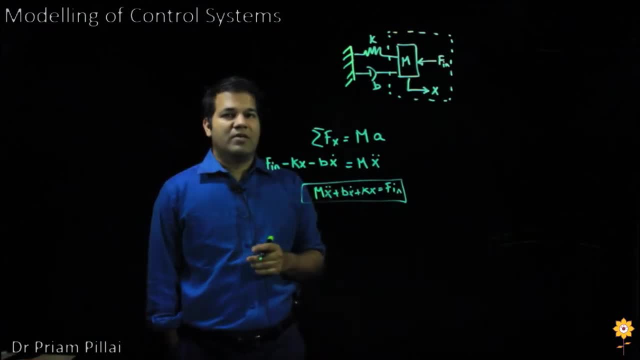 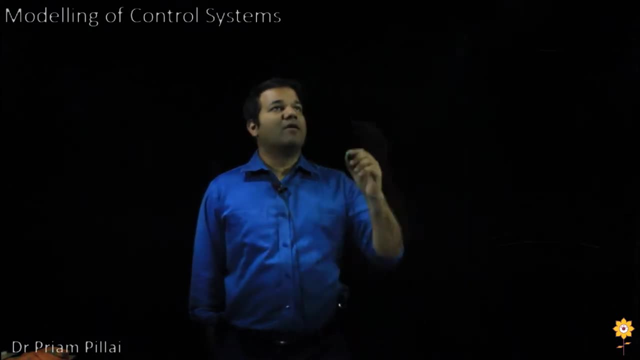 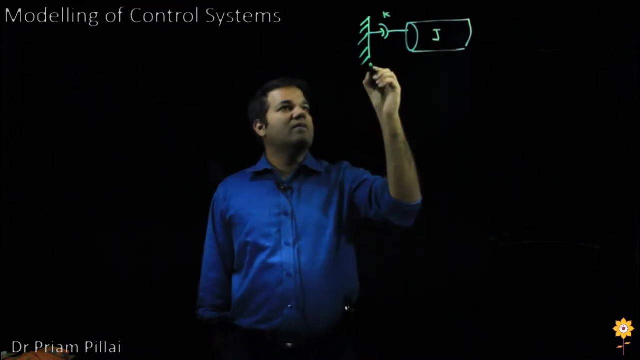 coefficients, and we'll discuss how to solve these in future lectures. Similarly, we can also consider a rotational mechanical system where, instead of a spring mass and a damper, we have a rotational spring, a shaft of moment of inertia J and a rotational damper, a rotational 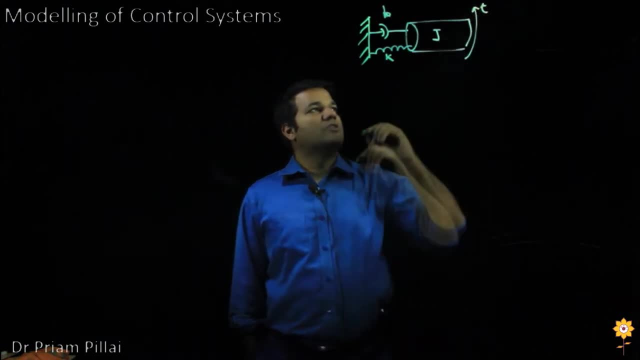 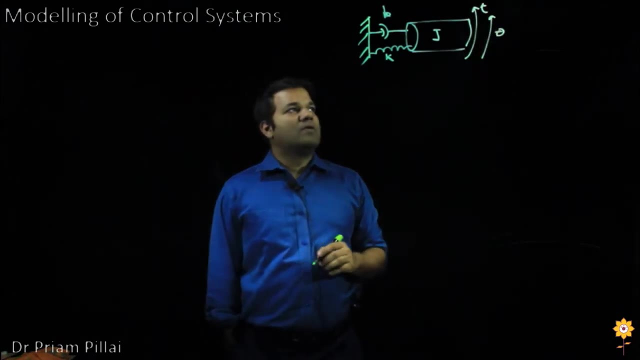 spring a shaft and we apply a torque on this shaft and we measure its angle as we rotate it. Thank you. The same way that we applied conservation of linear momentum, we can apply conservation of angular momentum here and to say that the sum of all the torques acting on that shaft 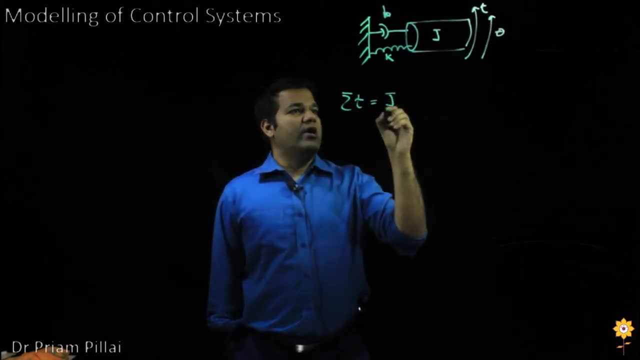 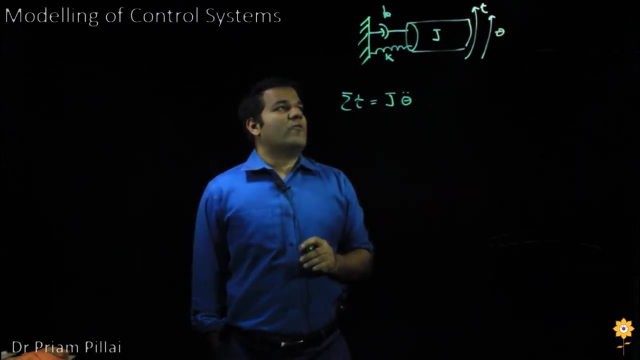 would equal the moment of inertia, J times the angular acceleration theta double dot. We can add up all the torques on that shaft and we'll get the input torque times the angular acceleration theta double dot. Now in minus the torsional stiffness multiplied by the angle, minus the damping multiplied. 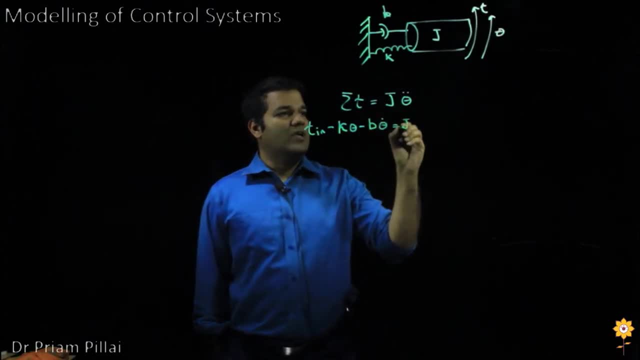 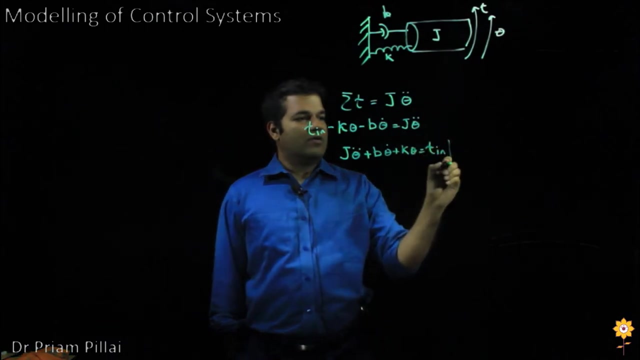 by the angular velocity of that shaft equals J theta double dot, and then J theta double dot plus B theta, dot plus K theta equals the input torque. Thank you, Thank you. Thank you, Mighty, helped with the talk Now. similarly, we have the same type of equation that we saw in the linear system or the linear 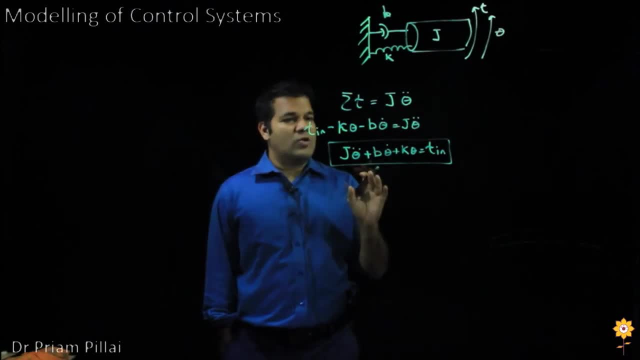 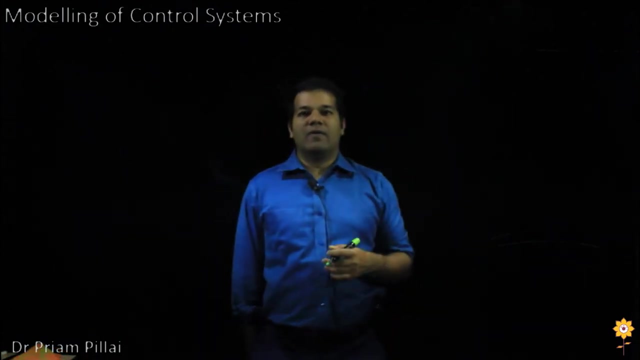 translational system. This system is also linear. It's a second order ordinary differential equation with constant coefficients. So you could envision that the solutions to this would look very similar to the solutions of the previous equations that we saw. Now let's also consider an electrical system. 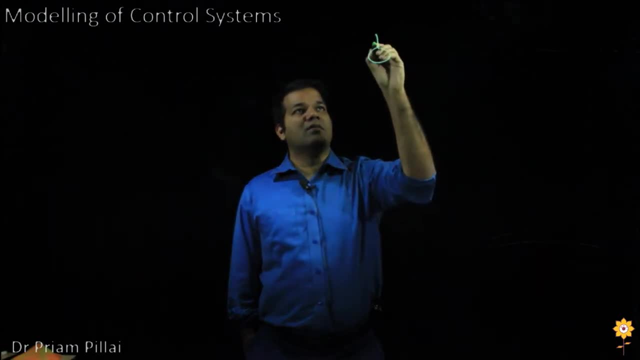 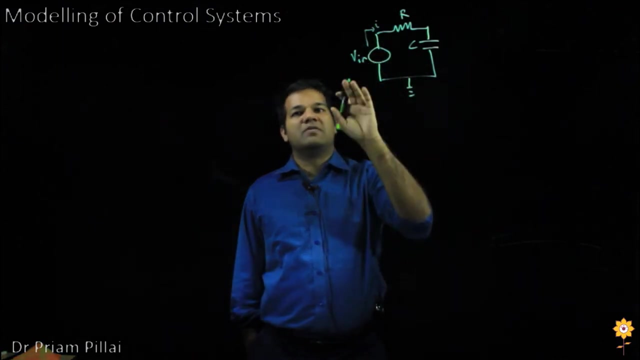 And in this case a simple RC circuit with an impedance minus 4.1 by 5.5.. Okay, with an input voltage V in a resistor R connected in series with the capacitor as the current I flows through it. our input is the voltage in and the output is the voltage across the. 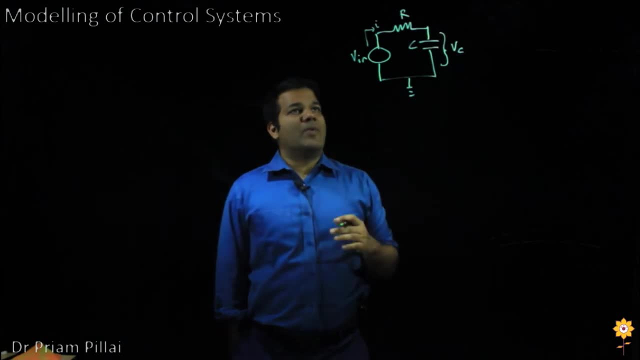 capacitor. We can also we can apply Kirchhoff's voltage laws to this circuit and what we end up getting is that V in minus V R minus V C, equal to zero, The sum of all the voltages along the circuit will be zero. So V in equals V C plus V R and V R as per Ohm's law will.